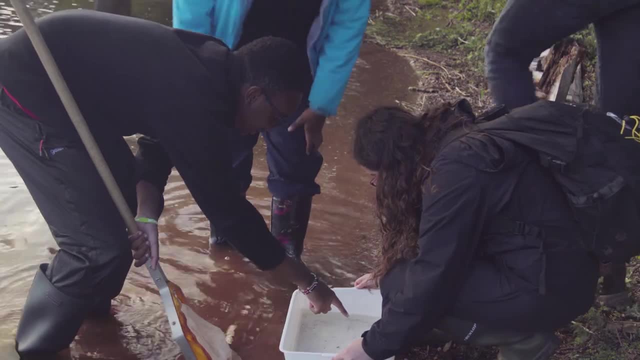 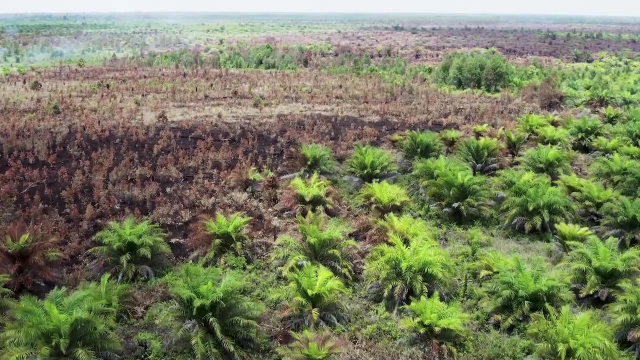 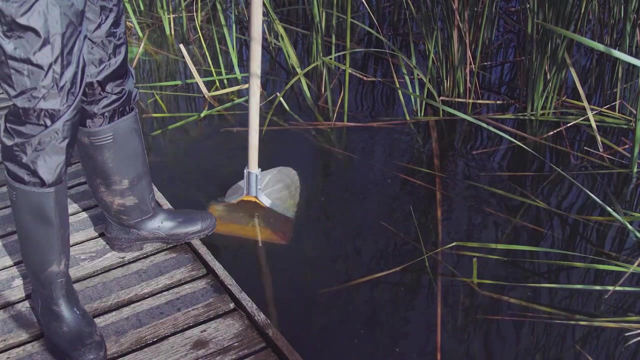 science programmes with a global reputation to gain the skills and knowledge needed to really do something about climate change And all the other environmental problems that humanity faces. Join thousands of graduates in over 30 countries around the world who are using the expertise they gained at Plymouth to really 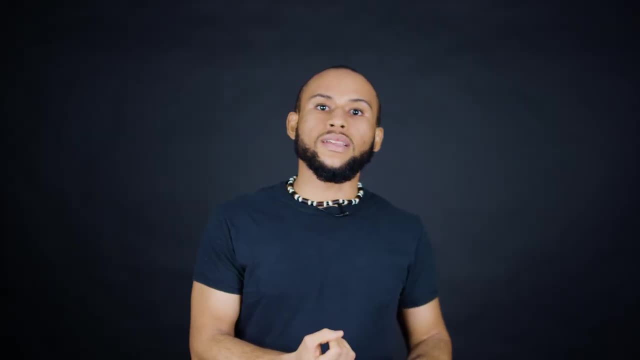 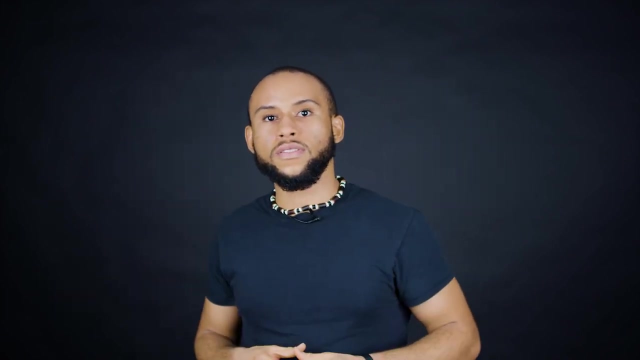 make an impact in saving this planet: BSc Environmental Science, BSc Environmental Management and Sustainability: Courses that matter, Courses that will make a difference. Remember: it's your future that's at stake. 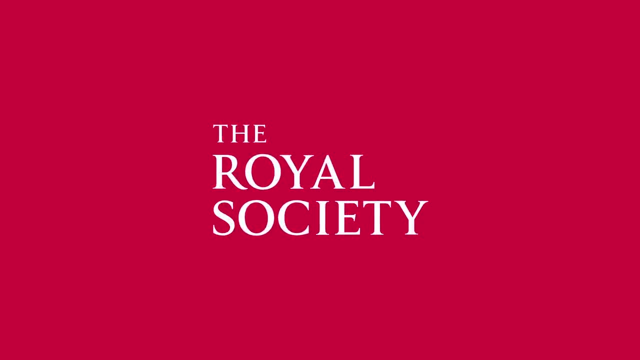 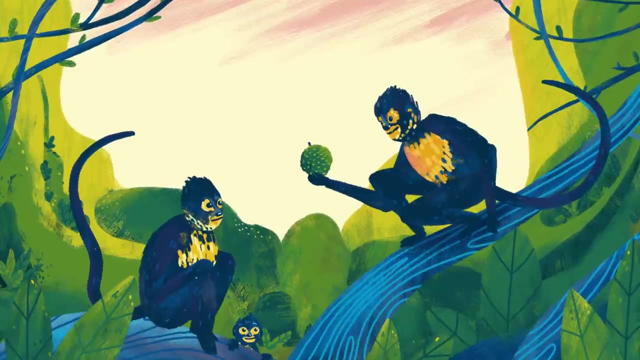 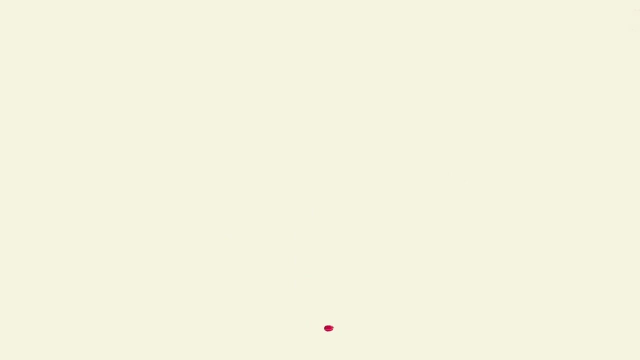 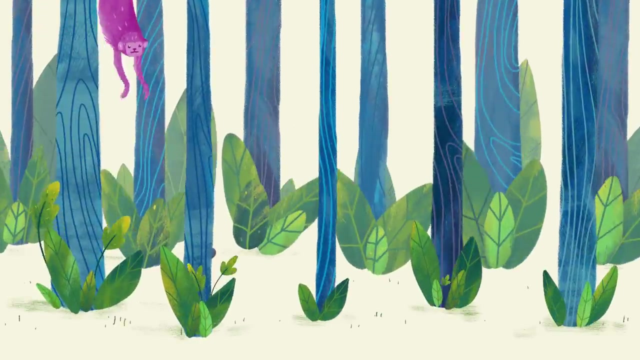 This spider monkey is an unwitting climate activist. Large fruit eaters such as this one spread the seeds of tropical hardwood trees in their dung, helping to build up forests which absorb carbon dioxide from the atmosphere. And this is just one of perhaps millions of. 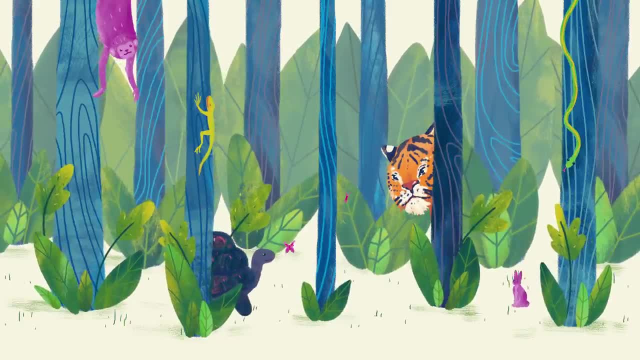 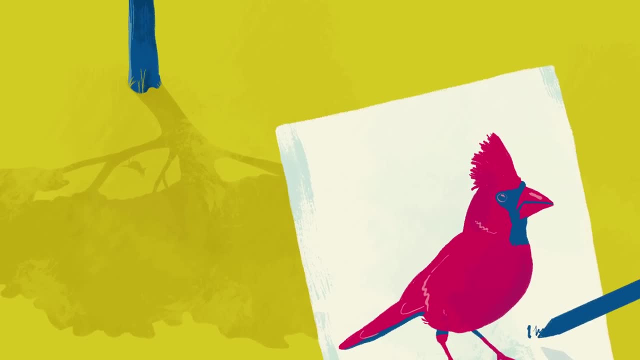 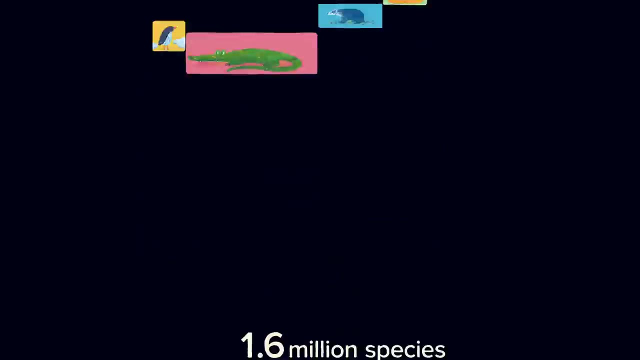 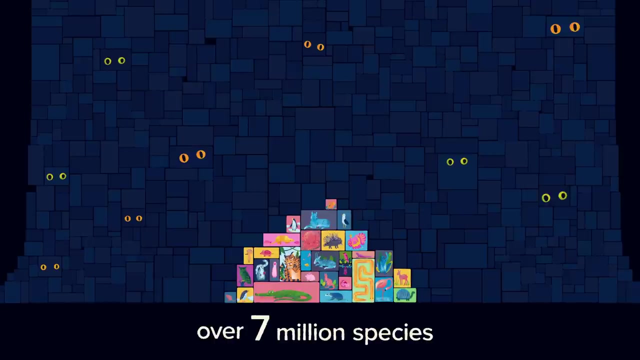 interactions that guarantee a healthy and functioning planet. Humans have spent hundreds of years documenting life on Earth, and we now have a catalogue of around 1.6 million species. However, there may be seven or eight million more that we don't yet know about. We have a 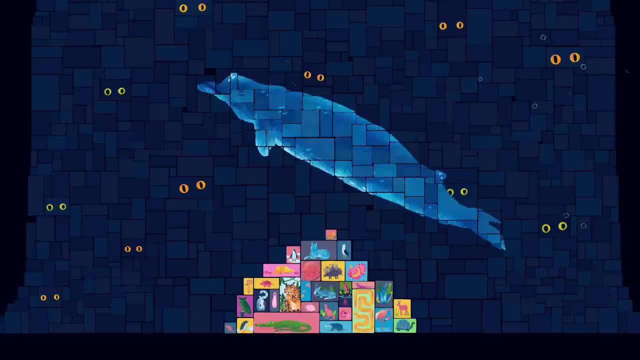 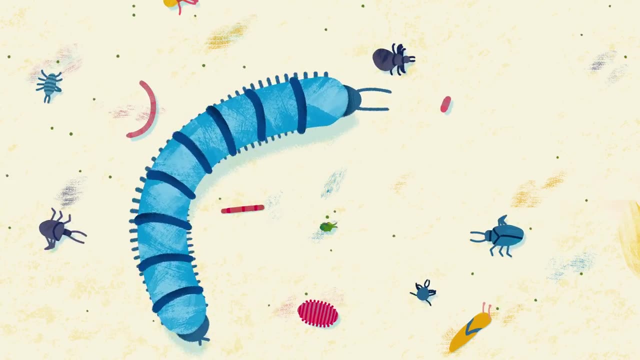 good idea of the large animals such as mammals and birds, but there are doubtless even some of these that we've missed, And the smaller you go, the more species there are left to find As the human impact on the planet intensifies. 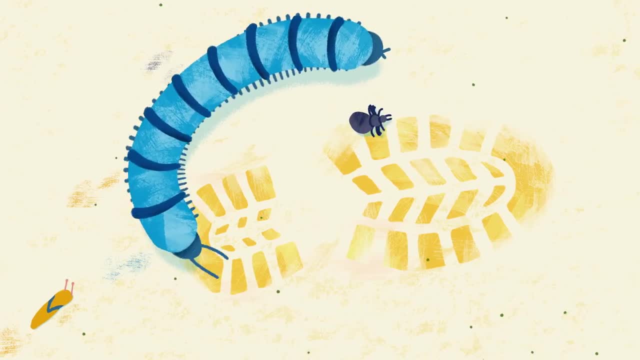 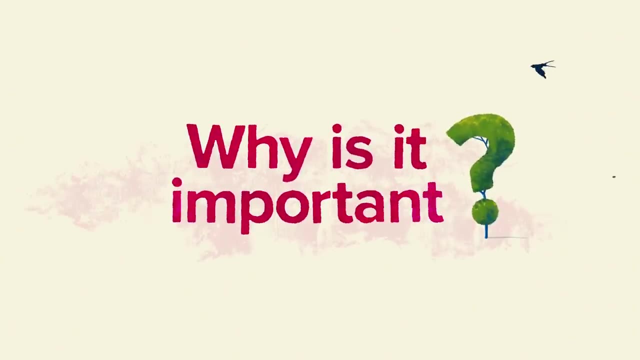 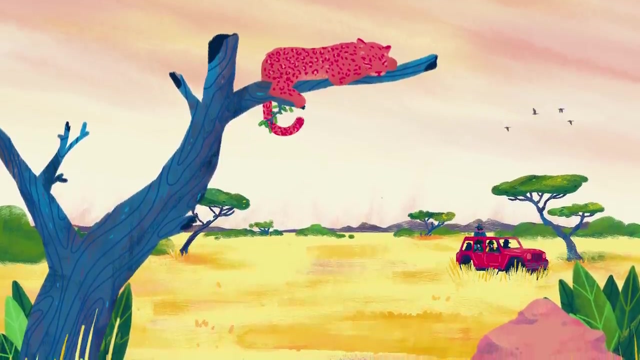 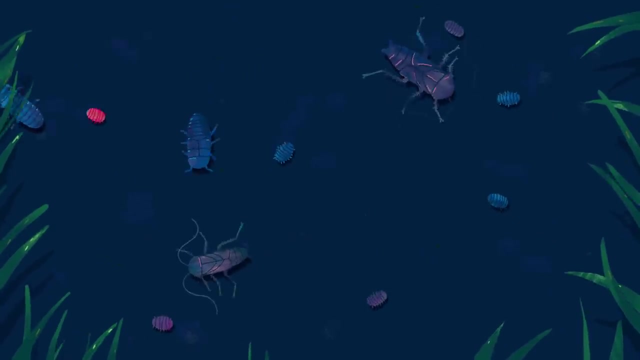 scientists fear that many species could be lost before we even discover them. So why is it so important that we protect our planet's biodiversity? When we think of protecting wildlife, we tend to picture the superstars, But the organisms that do most of the hard work keeping our planet healthy are the unglamorous ones This biodiversity provides us. 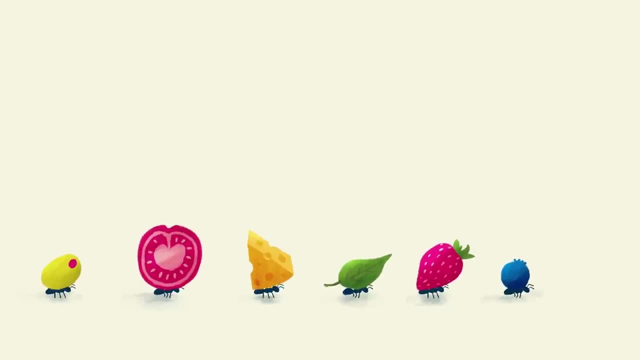 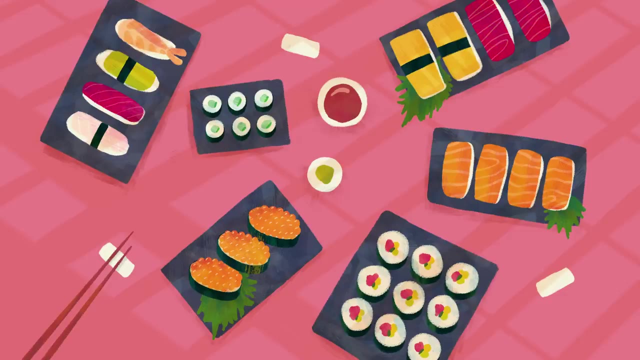 with the food we eat, from the microorganisms that enrich the soil where we grow our crops to the pollinators who give us fruit and nuts, and the fish that are the main source of animal protein for our food, And that's why we need to protect our planet. We need to protect our